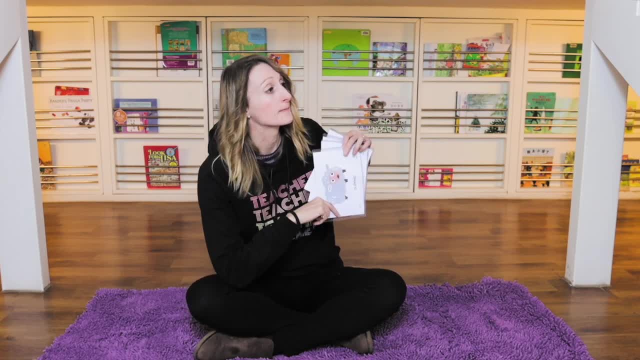 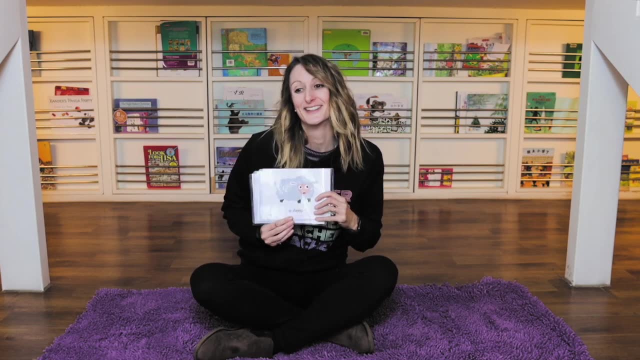 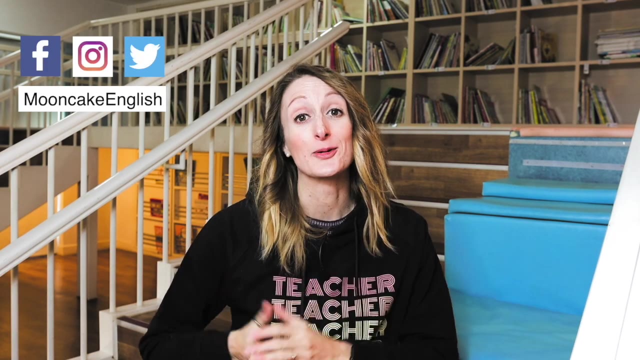 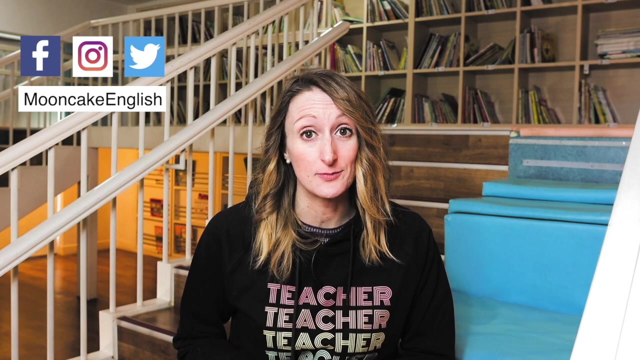 Yeah, yeah, I bought my flashcards Just so I just Hi. my name is Gemma Perry and welcome to Mooncake, where ESL teaching is made easy. If you're new here then you need to know that I make weekly ESL teaching tip videos to help. 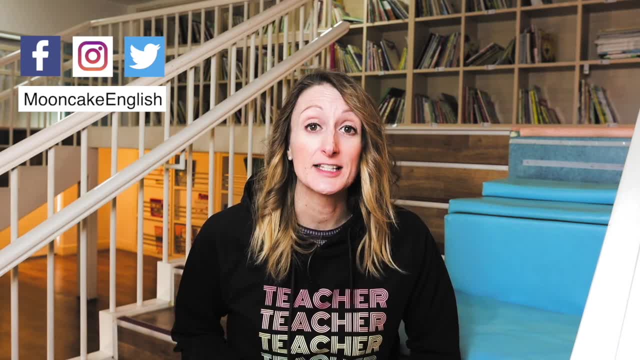 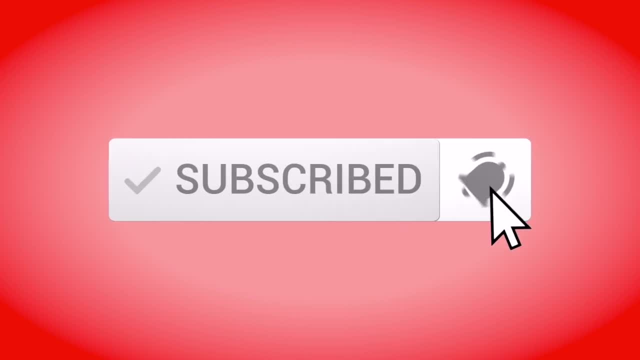 you improve your English teaching. So if you are teaching ESL online or abroad, make sure you subscribe below and hit that notification bell for weekly ESL teaching tips. Also real quick. if you are new here, say hi in the comments below and let me know where in. 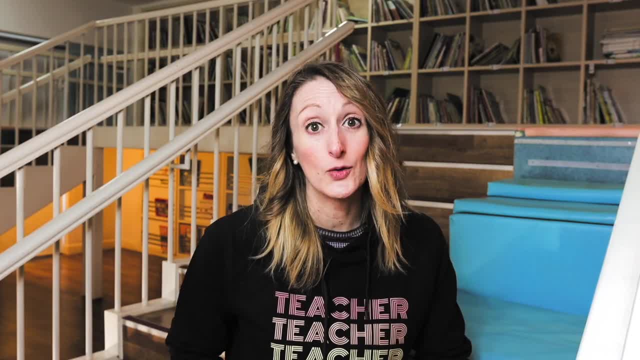 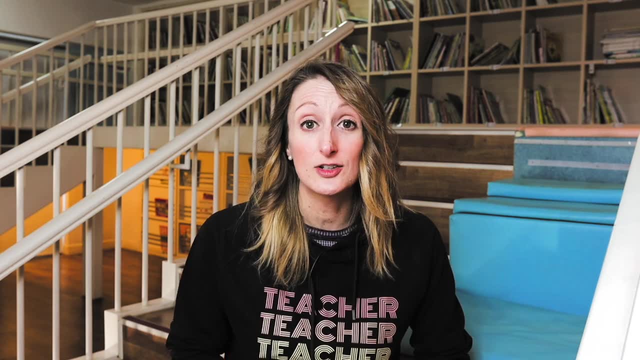 the world you're teaching. When you're a new teacher just starting out, it can be really tricky to know where to begin. Complicated flashcard games can be daunting, most especially if you're still learning how to manage your class successfully. But fear not, because today I'm 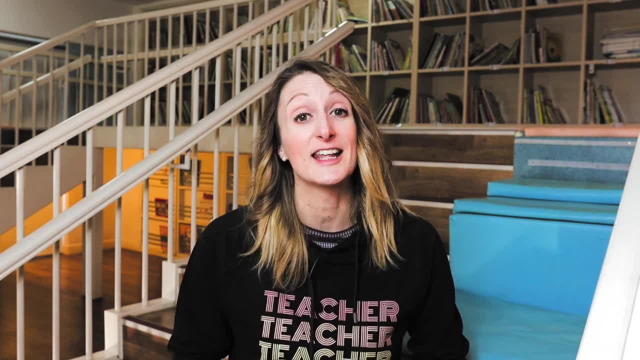 sharing with you how to manage your class successfully. But fear not, because today I'm sharing with you how to manage your class successfully. But fear not, because today I'm sharing five simple yet effective ESL games that every teacher should know. So, without further ado, let's get started. 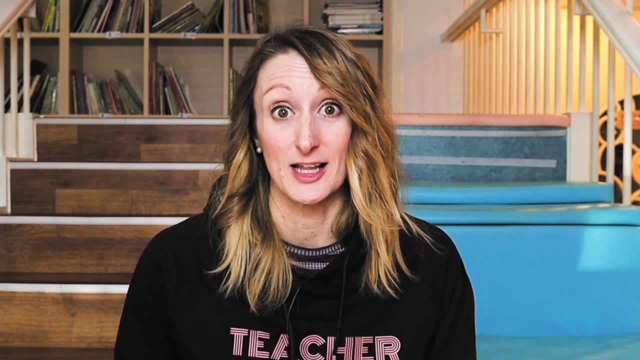 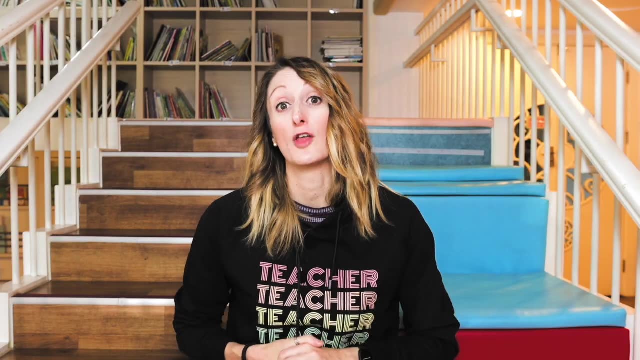 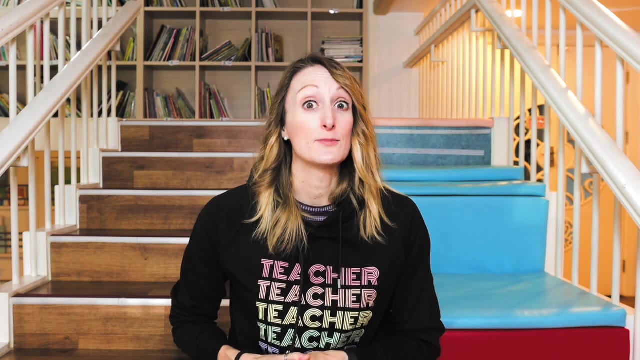 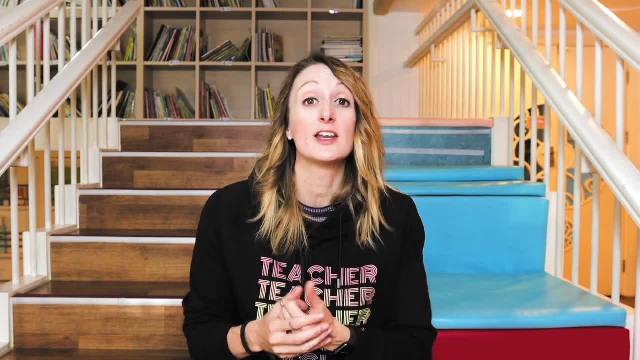 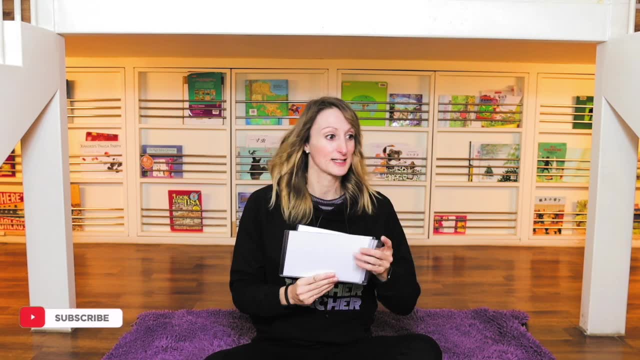 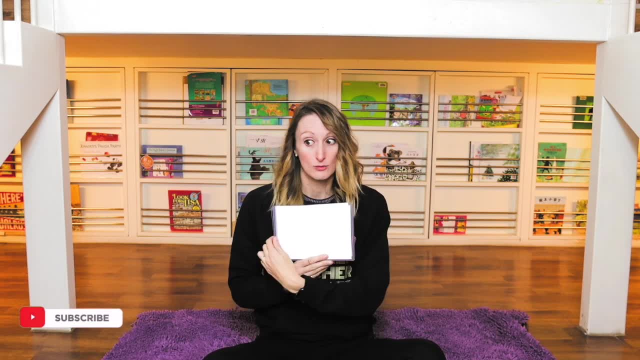 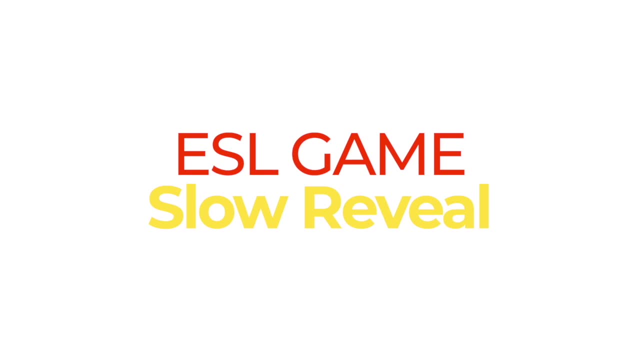 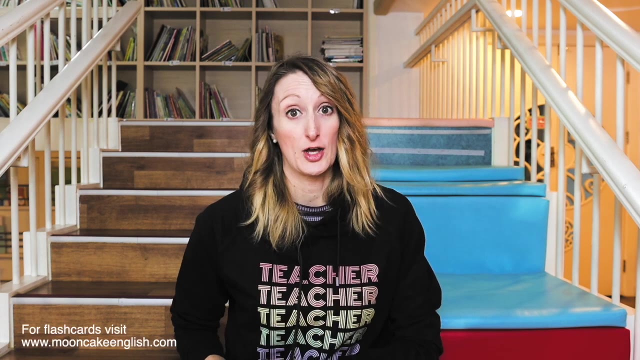 Are you ready? Three, two, one, What was it? What was it? This next game is called the Slow Reveal, and it's the complete opposite of the Quick Flash game. Once again, all you're going to need are some flashcards of the vocabulary that you want to. 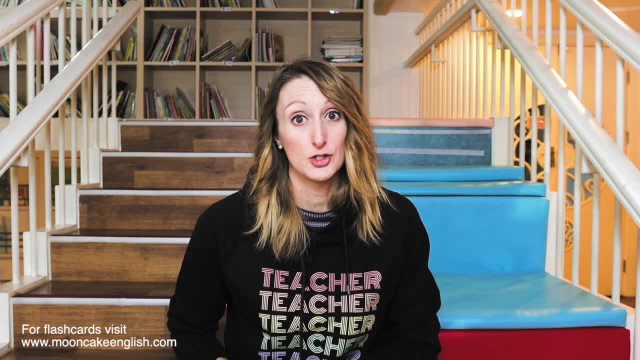 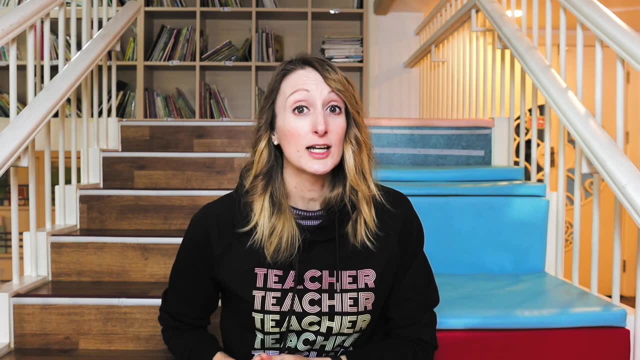 teach. Only this time. instead of quickly showing a flashcard to students, you're going to cover up the picture and slowly reveal it to students. Students then need to guess as quickly as possible what that picture is. With this game, you can reward points to the student that says the word the fastest. 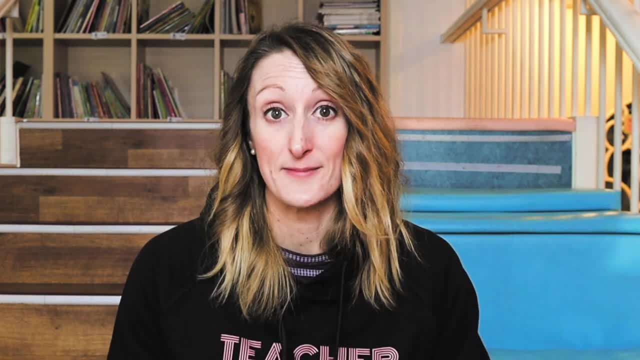 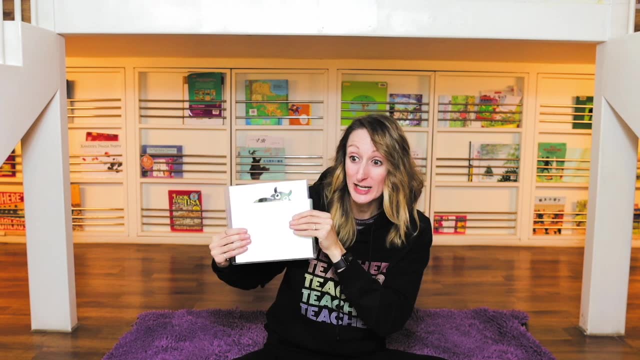 or split the class into two teams and turn it into a team game. What is it? Oh no, no, no, no, Guess what is it? What is it? What is it? Bing, bing, bing, bing, bing, bing, bing. 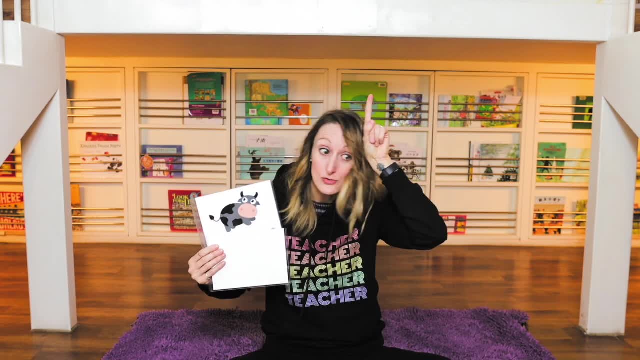 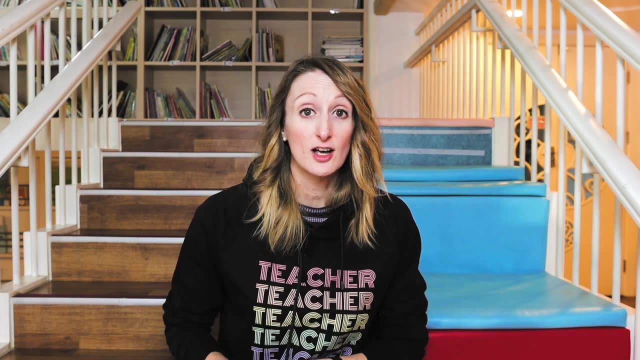 Good job. It's a cow moo moo. It's a cow moo moo. This next game is called Quieter Louder, and all you're going to need are some flashcards of the vocabulary that you'd like to teach. To get started, you're going to introduce one. 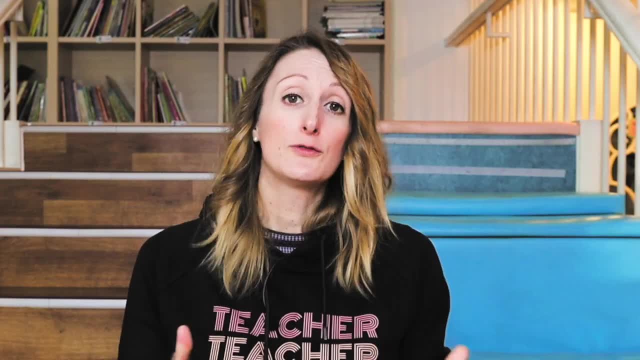 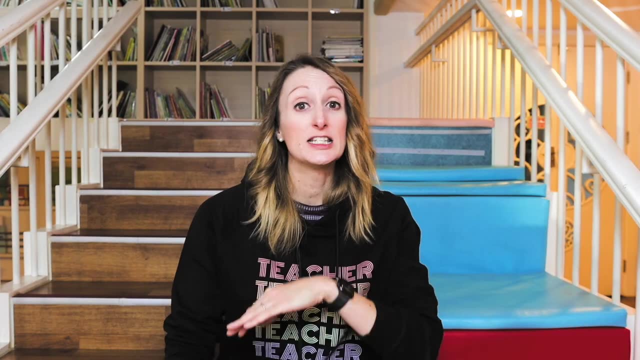 word to students using chance and TPR as you do. If you're not sure what I mean by chance and TPR, then make sure you check out my video on TPR linked below. Next, you're going to have students continue to repeat that word again and again as you move your. 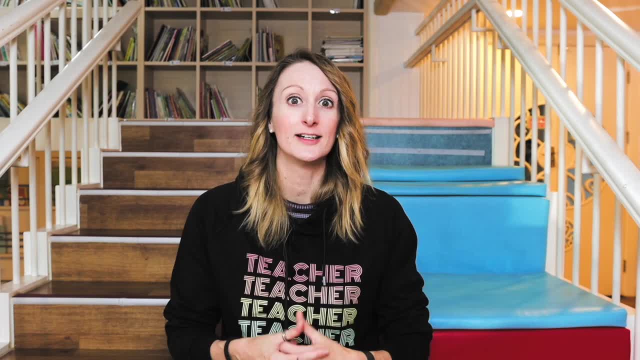 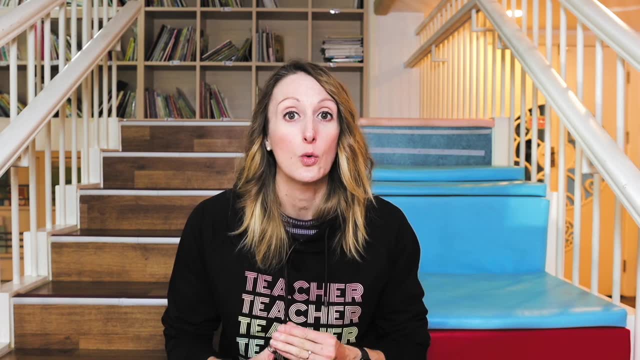 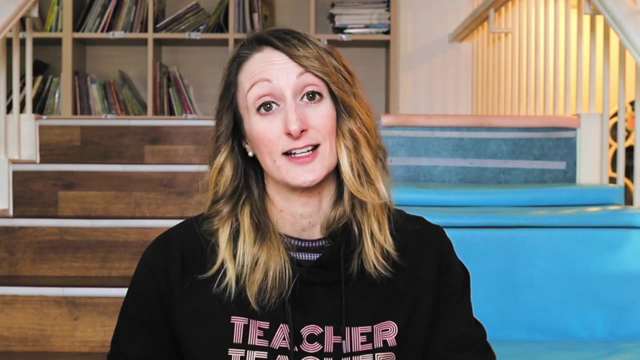 flash card up into the air, getting louder and louder as you do. Once you reach that peak, you're going to start moving that flash card downwards, getting quieter and quieter as you do. Remember to end this game on a quiet note so that it's easier to transition to the next activity. 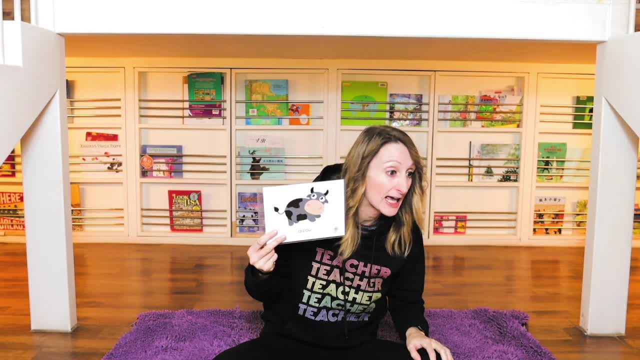 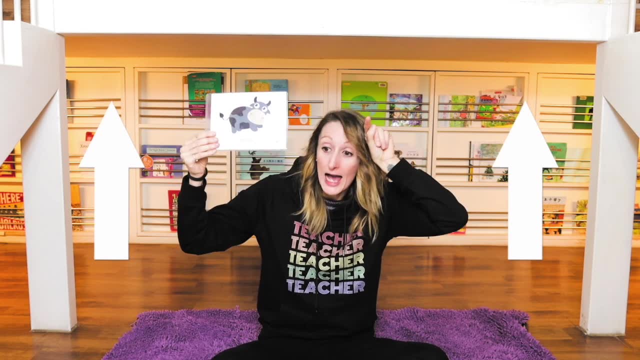 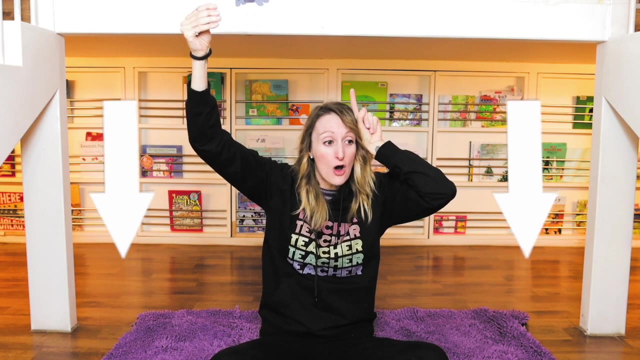 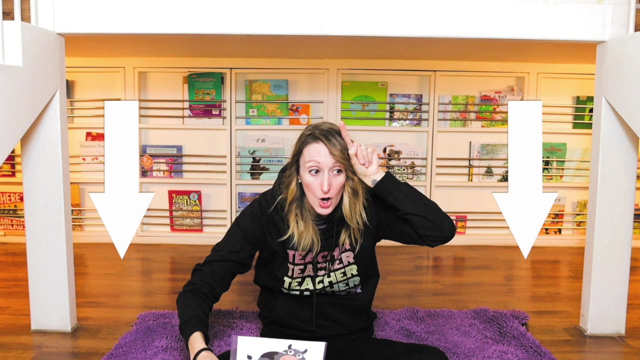 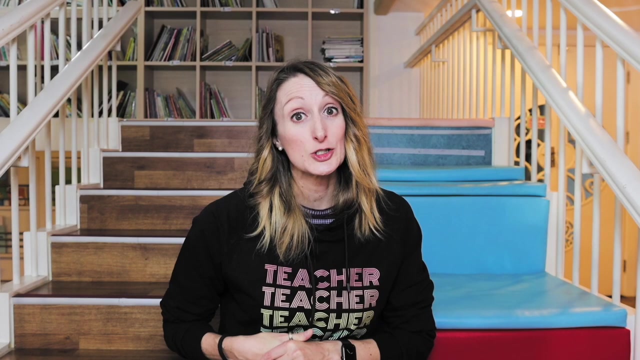 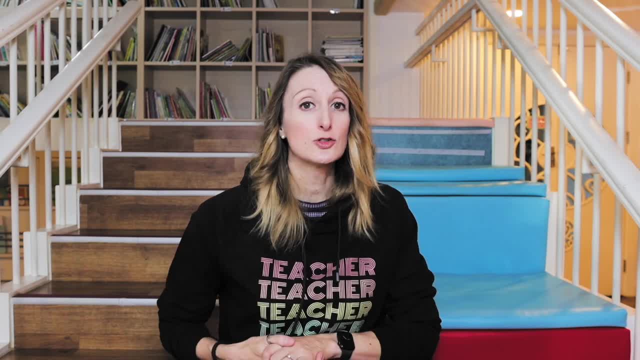 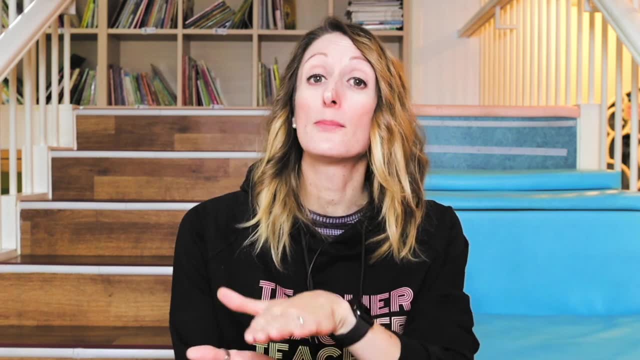 cards of the vocabulary that you want to teach. to get started, introduce the flash cards one by one, using chance and tpr as you do. next, you can lay those flash cards out face up on the floor in front of you and invite one student to come to the front. that student then needs to jump on the. 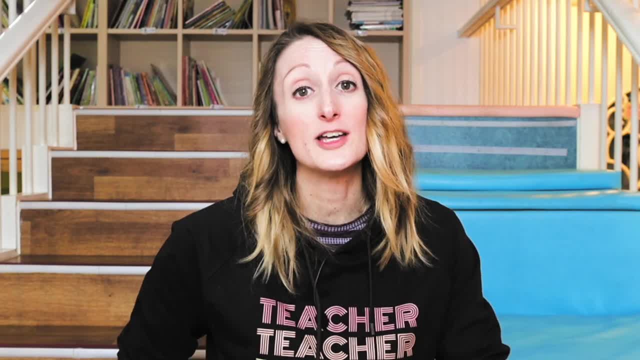 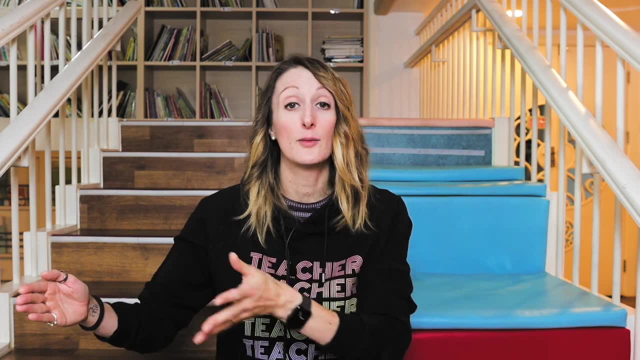 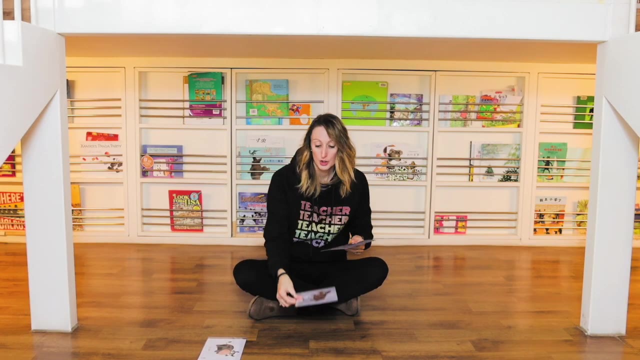 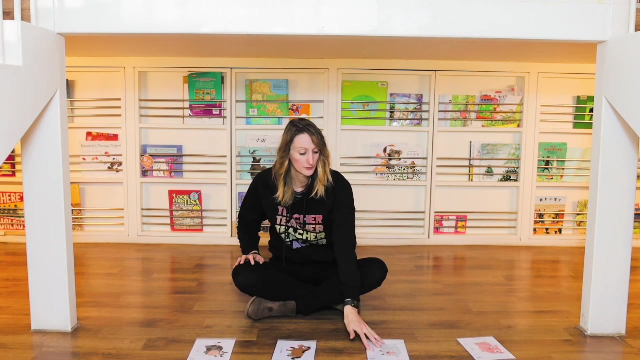 flash cards one by one, shouting out the word as they do. depending on your class size, you might want to have students come up one by one or have the whole class line up in front of the line of flash cards. think about your class and how best to manage it. one, two, three, four. one, two, three, four.